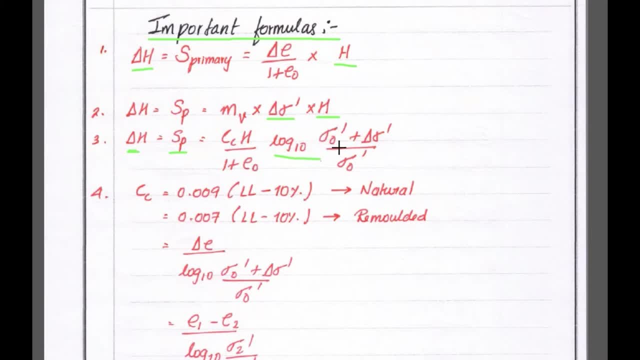 then sigma 0, dash equal to effective pressure and del sigma equal to change in effective pressure. Now the compression index formula, cc equal to 0.009 into liquid limit minus 10 percentage. So this is for natural condition. For remolded soil, the formula is equal to 0.007 into liquid limit minus 10 percentage. So now cc equal to another formula del e divided by log 10 sigma 0 dash plus e0 into h. So this is for natural condition. For remolded soil, the formula is equal to 0.007 into liquid limit minus 10 percentage. So now cc equal to another formula del e divided by log 10 sigma 0 dash plus e0, log 10.. So this is for natural condition. For remolded soil, the formula is equal to 0.007 into liquid limit minus 10 percentage. So now cc equal to another formula del e divided by log 10 sigma 0 dash plus e0, log 10.. So this is for natural condition. For remolded soil, the formula is equal to 0.007 into liquid limit minus 10 percentage. 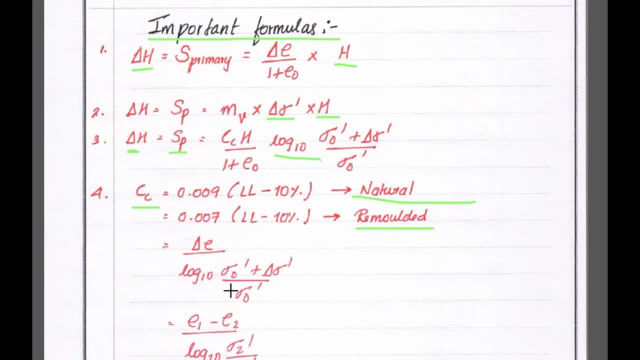 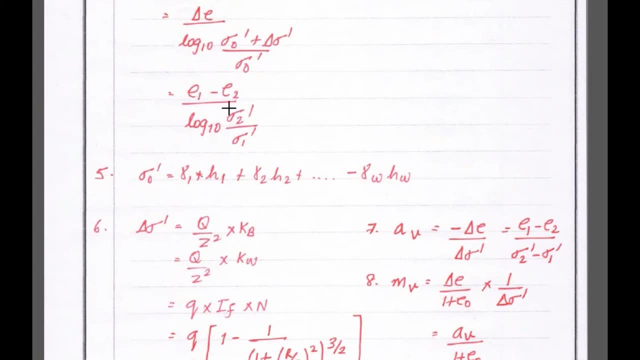 So this is for natural condition For remolded soil. the formula is equal to 0.007 into liquid limit minus 10 percentage. So this is for natural condition For remolded soil. the formula is equal to 0.007 into liquid limit minus 10 percentage. 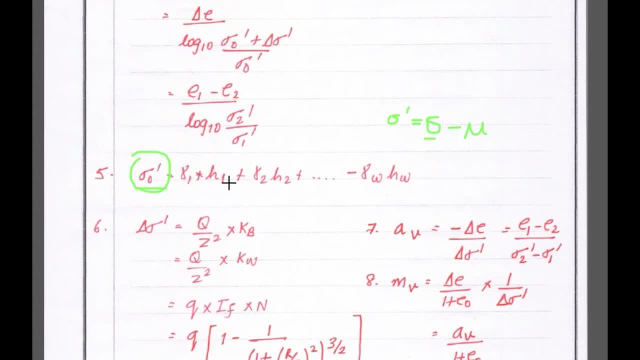 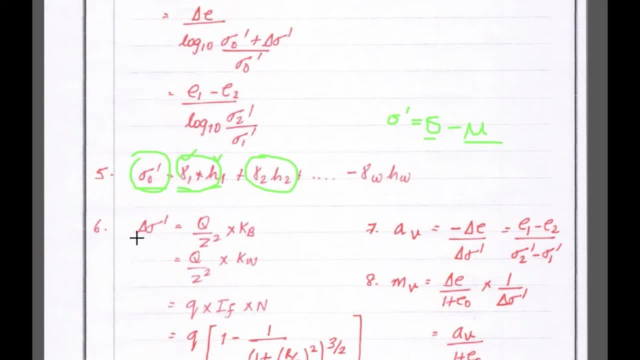 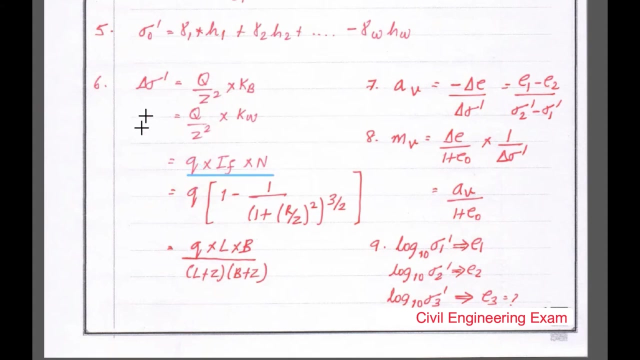